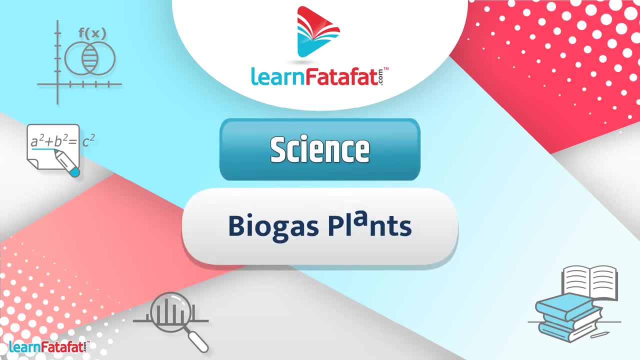 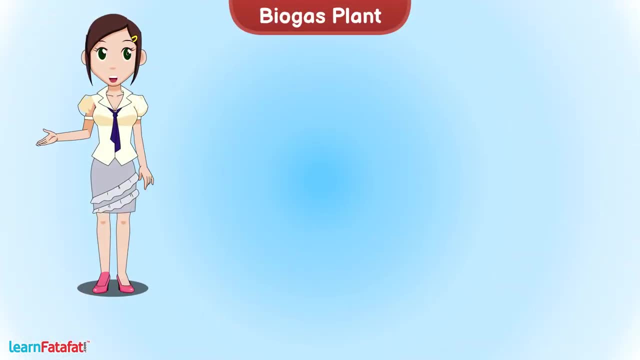 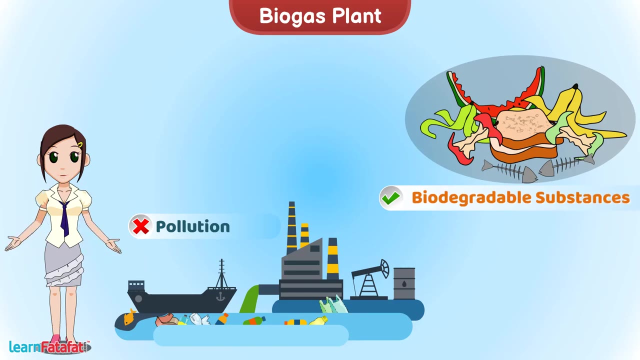 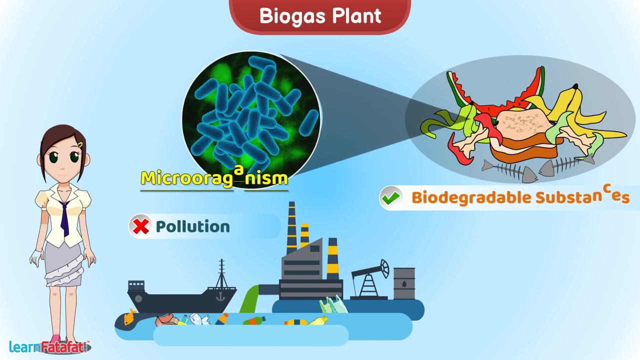 Today, we will learn about biogas plants. Many times we have heard that, in order to reduce pollution, we should use biodegradable substances. Do you know the reason behind this? Yes, the biodegradable substances are decomposed by microorganisms and hence these do not cause pollution. 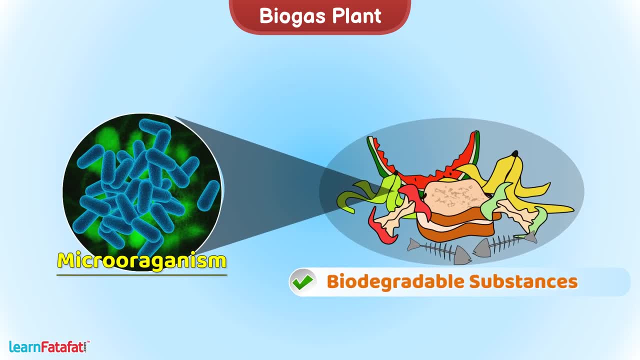 But when these biodegradable substances are decomposed by anaerobic microorganisms, in absence of oxygen, the methane gas is released. That's why this anaerobic decomposition is called biodegradable. This decomposition process is used for the production of methane gas by the biogas plants. 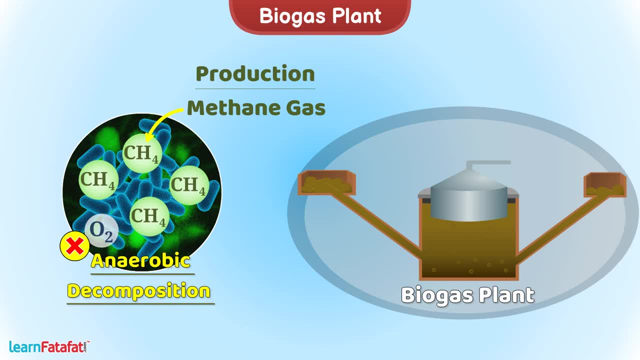 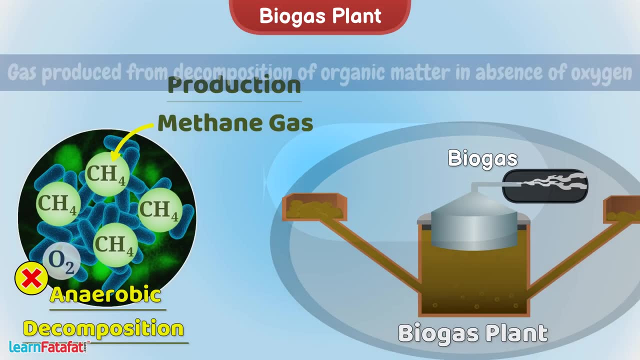 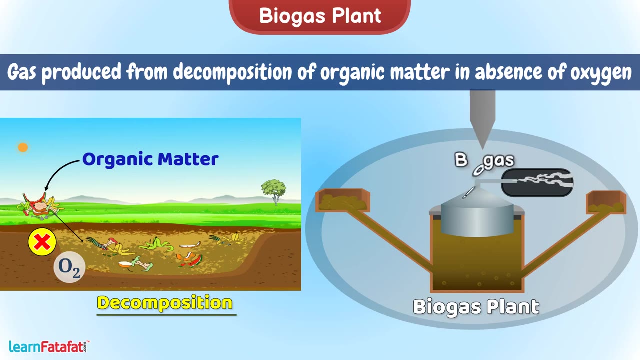 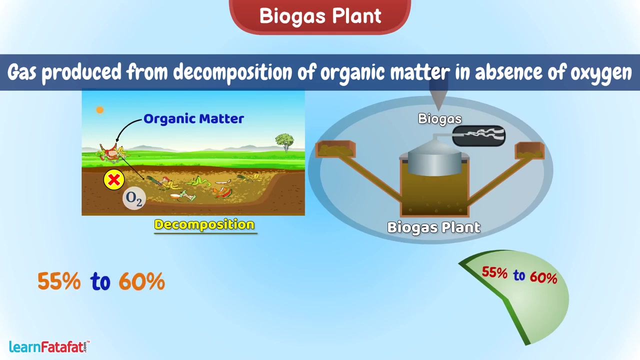 Let's know about it. A biogas plant is a plant in which the biogas is produced. The gas produced from the decomposition of organic matter in absence of oxygen is called biogas. Biogas consists of 55% to 60% methane and the rest is carbon dioxide. 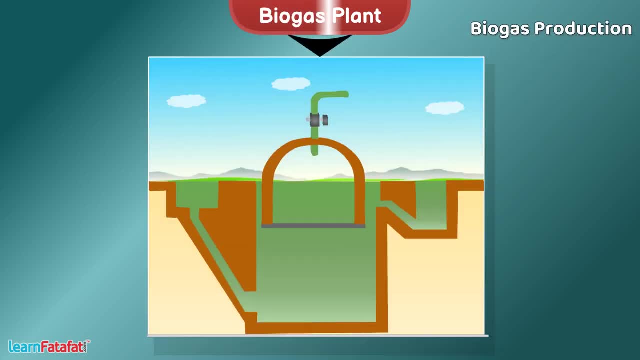 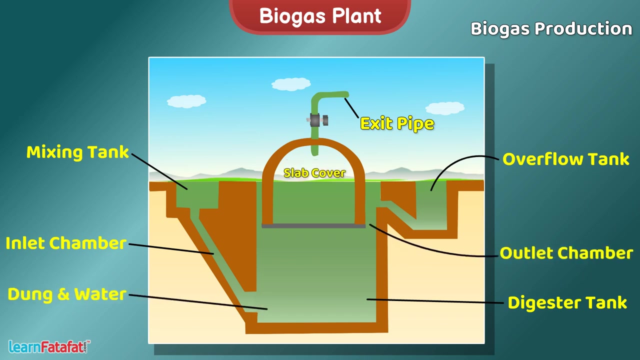 The biogas production is carried out in biogas plants. It has five components: A mixing tank, an inlet chamber, a digester tank, an overflow tank and an exit pipe For production of biogas. the biogas plant is produced by the biogas plant. 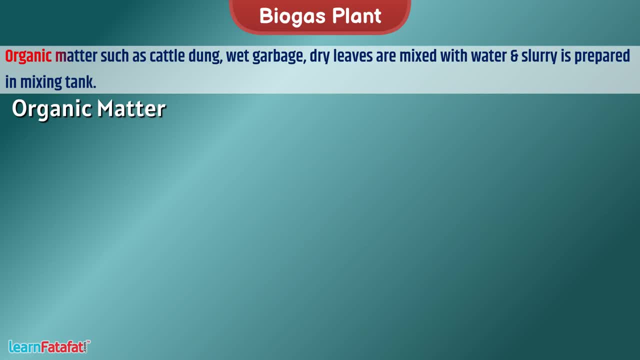 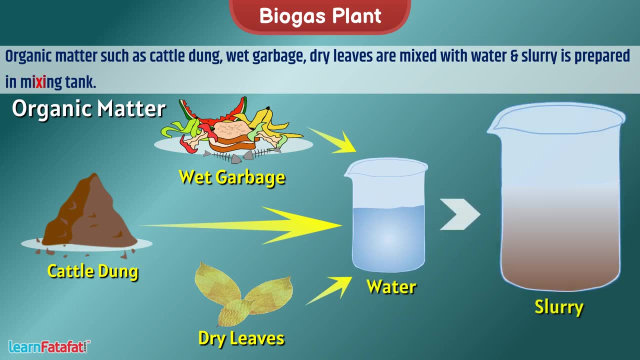 For production of biogas. the biogas plant is produced. by the biogas plant For production of biogas, organic matter such as cattle dung, wet garbage, dry leaves are mixed with water and slurry is prepared in a mixing tank. 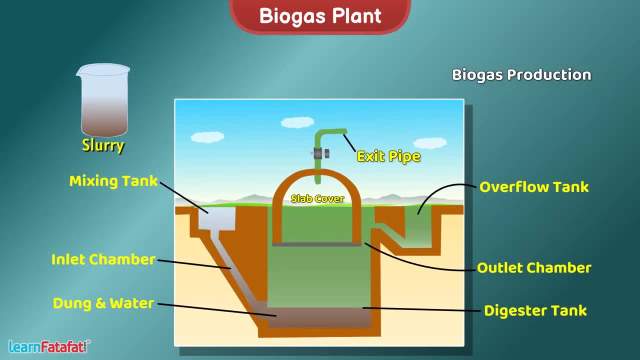 Through the inlet chamber, the slurry is feeded into the digester tank, where the actual process takes place in two steps. First, the microorganisms act on the complex biodegradable. Second, the microorganisms act on the complex biodegradable. 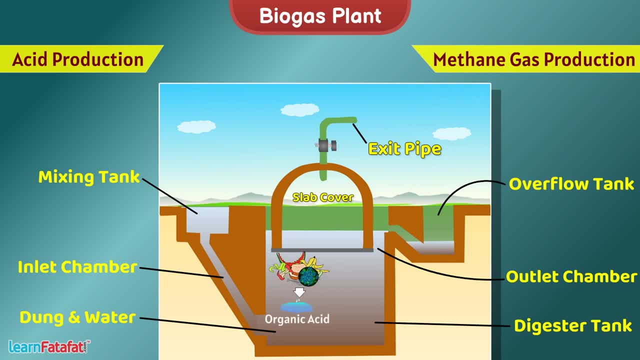 Third, the microorganisms act on the complex biodegradable. Fourth, the biogas plants produce biodegradable organic matter and produce organic acids. After this, the methanogenic act on the organic acid and produce methane gas, ie biogas.